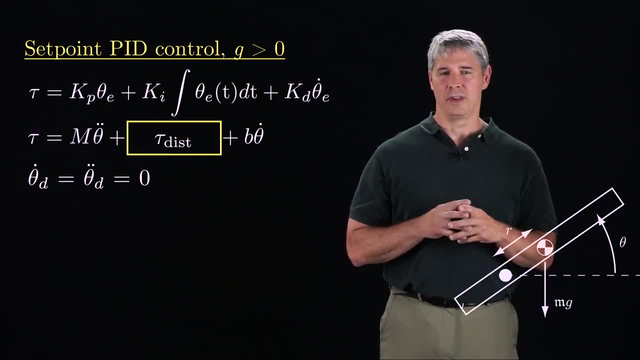 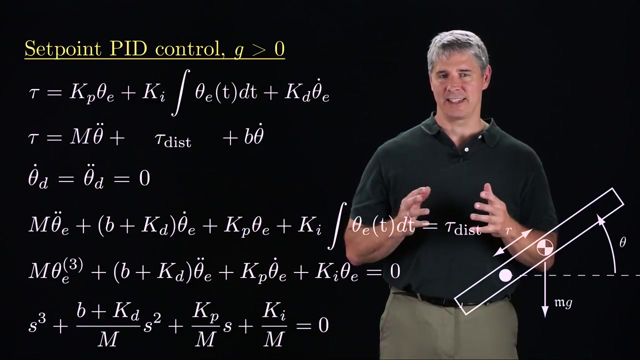 I'll be considering the steady-state behavior of the controlled robot when this non-linear term approaches a constant. Equating the dynamics in the control torque, we get the error dynamics. To get a differential equation, we can differentiate both sides. The result is a homogeneous third-order differential equation with this characteristic equation. By adding an integral term to the controller, we added a state to the dynamics. 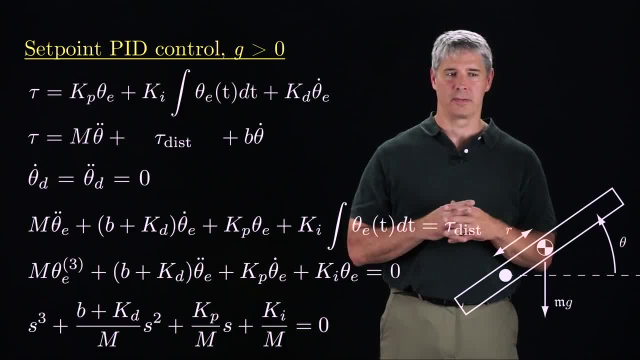 For stability, the roots must all have a negative real component. As for the PD controller, 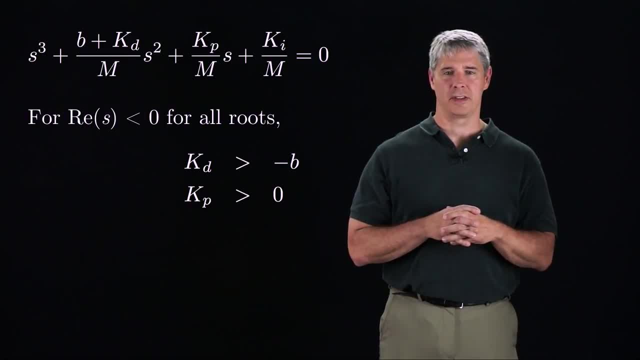 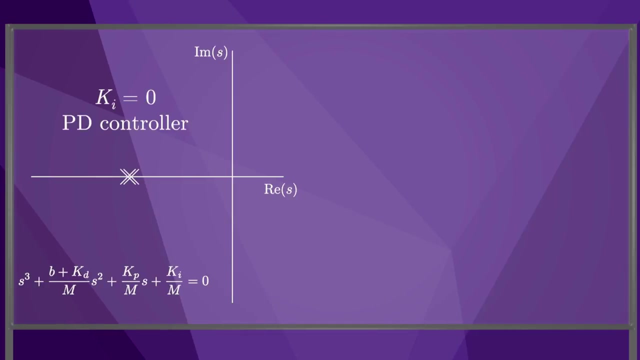 KD must be greater than minus B, and KP must be greater than zero. The gain KI must also be greater than zero, but, unlike KP and KD, KI also has an upper bound for stability. Before, for our second-order differential equation, the only dangers in choosing large gains were due to practical considerations. Like actuator limits, unmodeled dynamics, and finite servo frequencies. Now with a third-order PID-controlled system, even our ideal linear model shows that choosing KI too large could result in instability. Let's see this graphically by plotting the roots in the complex plane. First, let's choose KI equal to zero and choose the gains KP and KD to give critical damping, two collocated roots on the real axis. We'll keep KP and KD constant. We'll keep the roots in the complex plane, and the roots in the real axis. KD will give 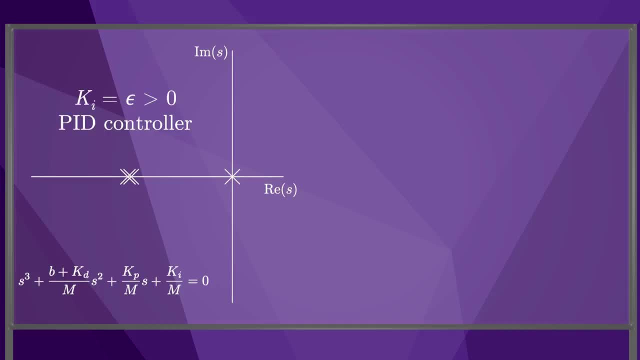 Next, let's add a small positive Ki. This creates a third root close to the origin. 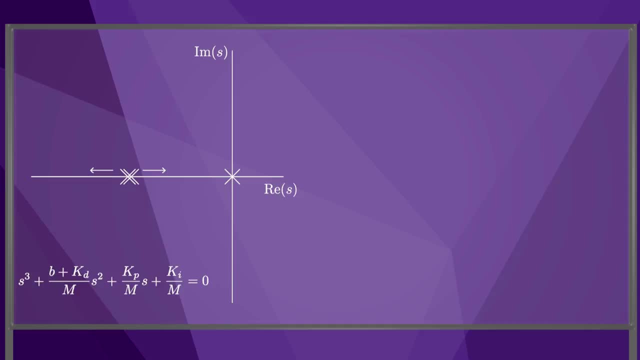 As we increase the gain Ki, the two co-located roots move away from each other on the real axis, and the root at the origin moves left. 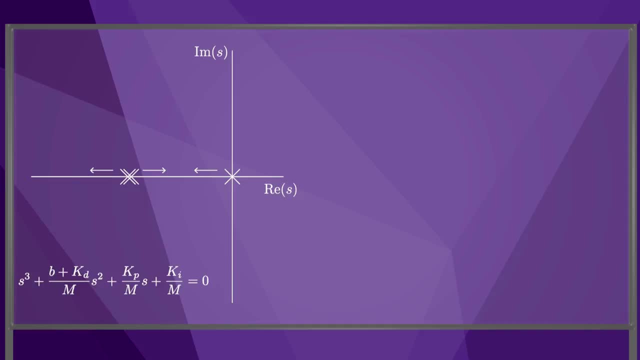 When we've increased Ki sufficiently, the two roots meet on the real axis, while the third has moved further left. Since the two co-located roots are much slower than the root far to the left, the transient 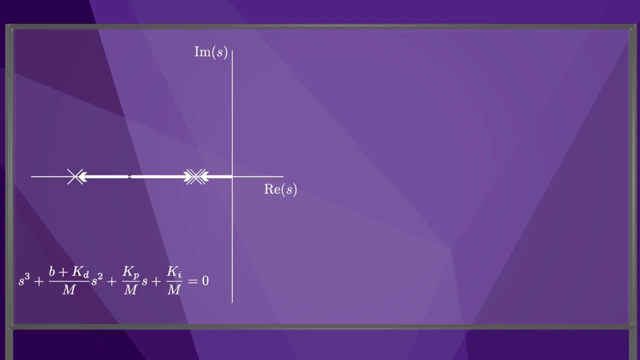 error response of this third-order system is similar to that for a critically damped second-order system. 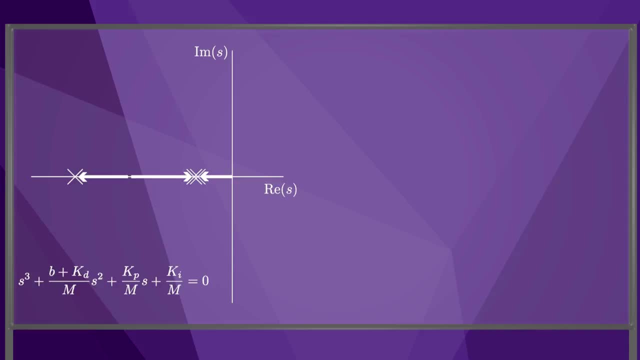 The response is slower than for the original critically damped PD controller, though, because the co-located roots are now further to the right. 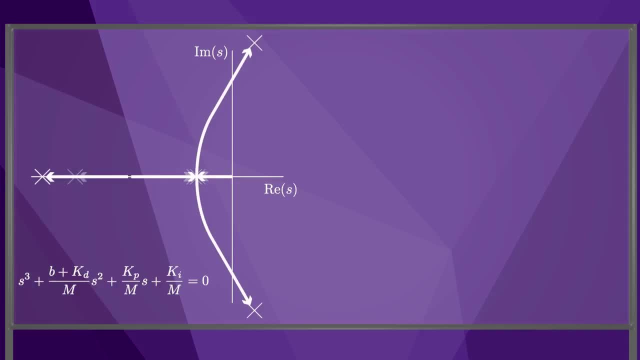 If we continue to increase Ki, the two co-located roots break away from the real axis and move into the right half-plane when Ki reaches its upper bound for stability. 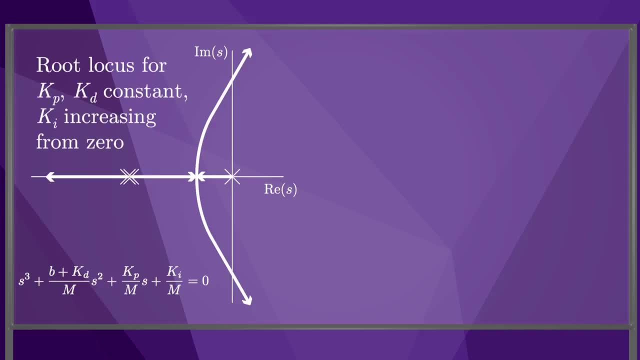 The error dynamics would be unstable for the roots shown. We've drawn the root locus for Ki. We can see that Ki is increasing from zero, and it demonstrates the key features of adding integral control. The integral term can improve steady-state response, but it can worsen the transient response. 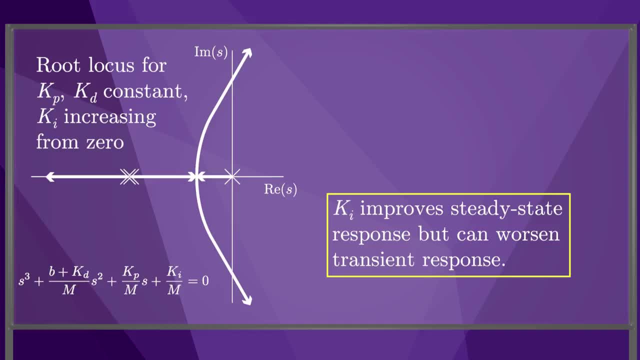 In particular, adding an integral term could cause overshoot and oscillation, and in the worst case, instability. 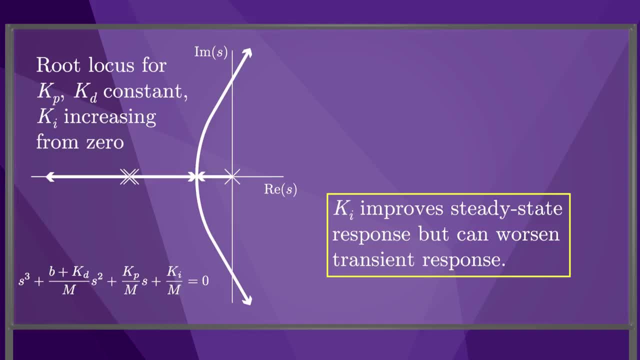 Since stability is paramount in control, often robot controllers avoid the use of an integral term, prioritizing stability over steady-state error reduction. Or if a non-zero gain Ki is used… 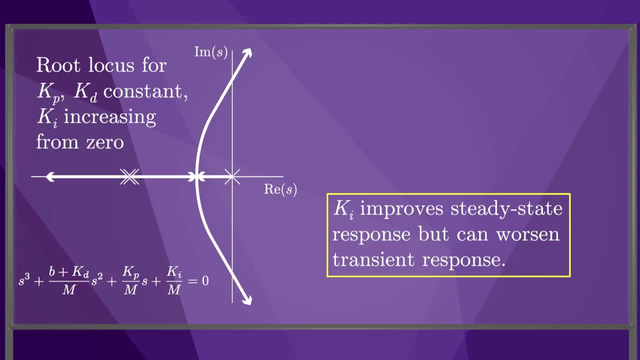 …it is chosen to be small. In addition, the magnitude of the integrated error may be capped at a maximum value. 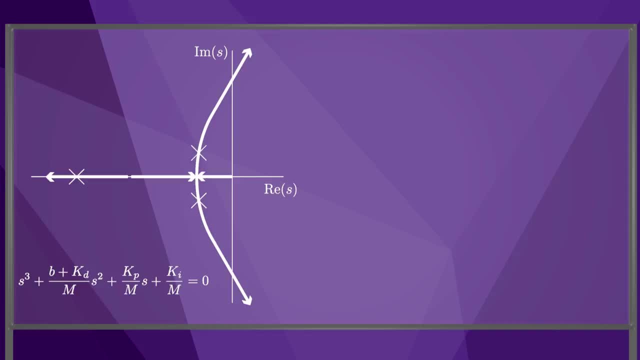 Let's design our PID controller to place the roots as shown here, which will yield an under-damped error response. 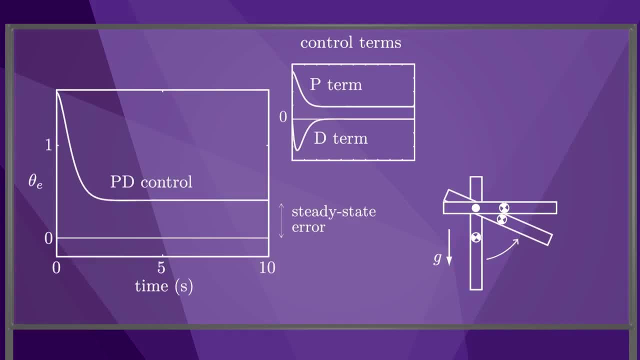 Returning to our example set-point control problem, we recall that our original PD controller 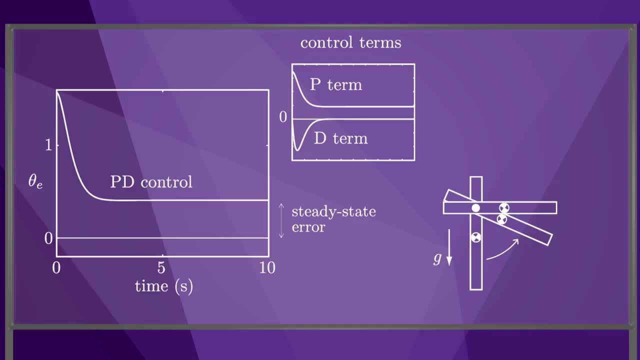 results in steady-state error. Adding a positive gain Ki, we see that the PID controller drives the steady-state error to zero. 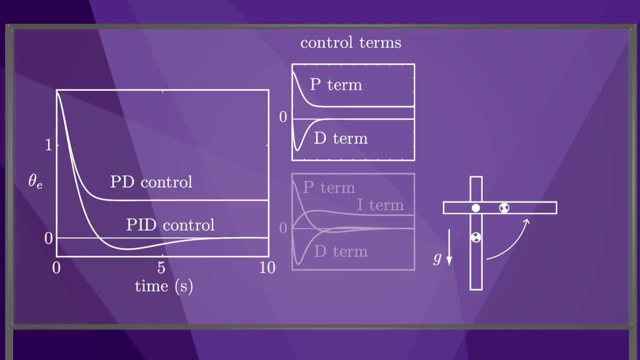 The overshoot shows that the response is somewhat stable. The PID controller is somewhat under-damped. Examining the torques due to the proportional, integral, and derivative terms, we see that the proportional and derivative terms both go to zero, while the integral term reaches a non-zero steady-state. 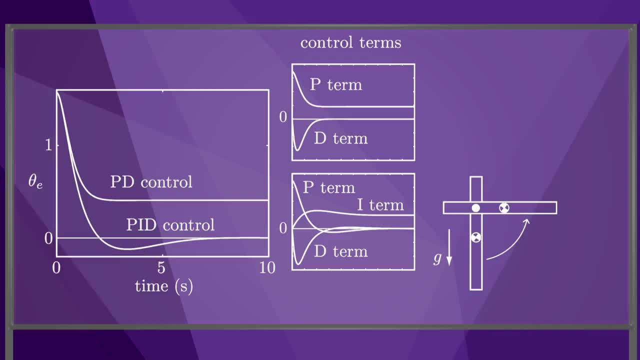 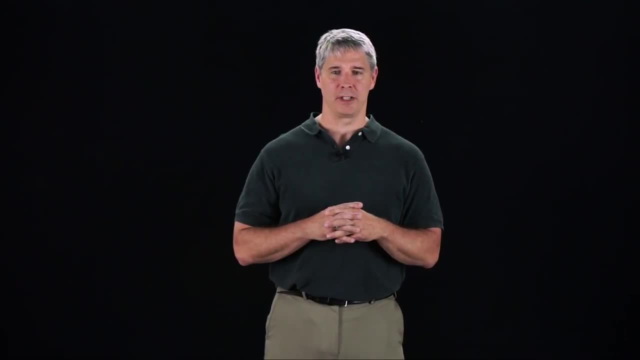 That is the torque that allows the joint to resist gravity even when the error is zero. In the next video, we'll combine PID feedback control with a dynamic model of the arm to derive our gold standard motion controller, the computed torque controller. Thanks for watching. We'll see you next time. Bye.